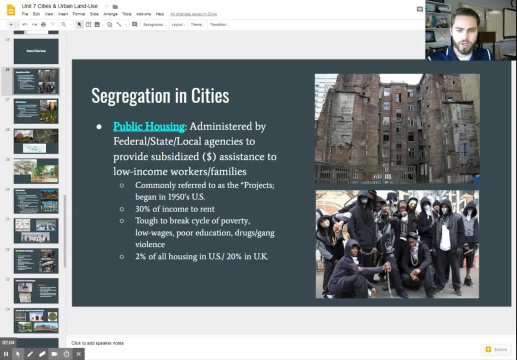 wouldn't get fixed. You had people in there that obviously didn't make a whole lot of money, and so oftentimes, when people don't make a whole lot of money, they turn to some less than above board practices, such as, you know, drug dealing and gang violence and many other bad associations with. 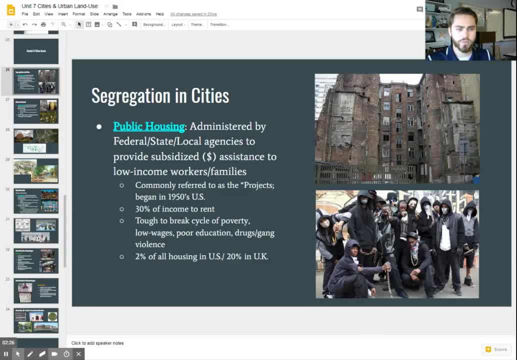 public housing, And so that's where they get the term the projects or the ghetto, because of these dilapidated buildings and the crime rates that are associated with the public housing. So what intended to be a good thing for the city and for its less fortunate residents ended up becoming areas of the city that 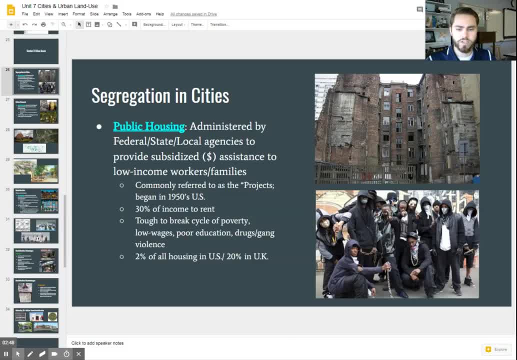 became very hostile and heavy crime and heavy poverty in that area, And so we see a lot of public housing as a big problem. We start seeing, you know, the areas become really run down and businesses don't want to put their businesses there anymore. They want to move to the nicer. 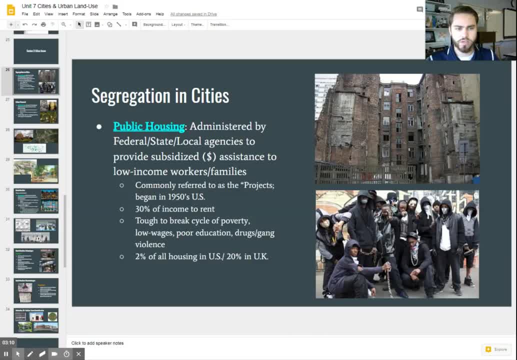 areas of town where there's not public housing, And so this creates this cycle of poverty in this particular areas of the cities, And what we tended to notice was that a lot of the people in these public housing were minorities, Usually people of African American or Hispanic descent, And so it 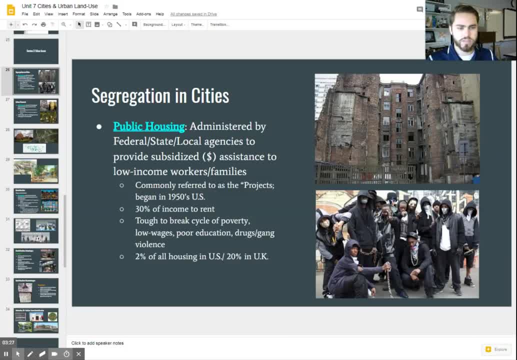 the cities in many ways that the white residences did not want to be near the public housing, so they would move to other parts of the city or eventually to the suburbs to get away from these public housing complexes, and you know so. this is one reason that we still see segregation in cities today, if you look 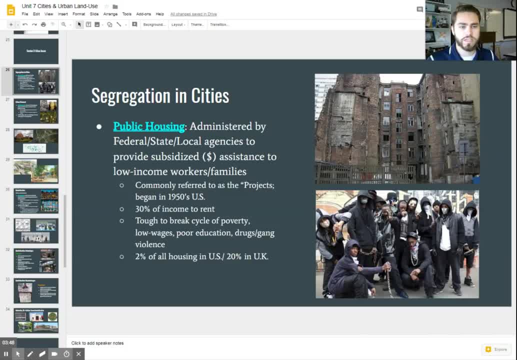 at a population map of many cities. it's still very segregated, based on, you know, racial or ethnic lines. so what intended to be a good thing from the government ended up becoming a major problem, and why we have certain areas of towns that are considered bad or heavy crime areas and- and that's still true today- all 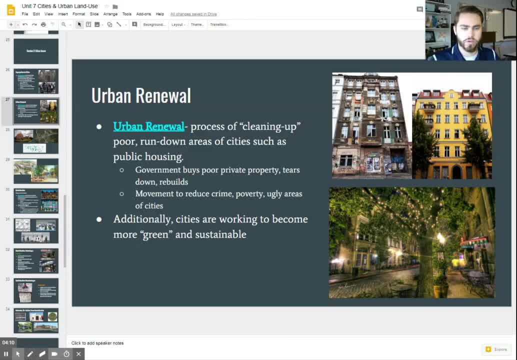 right. so what the government is trying to do now is what they call urban renewal. this is the process that they are buying up a lot of these properties and trying to fix them up, clean them up, you know. move the public housing, you know. move the public housing, you know. move the public housing, you know. 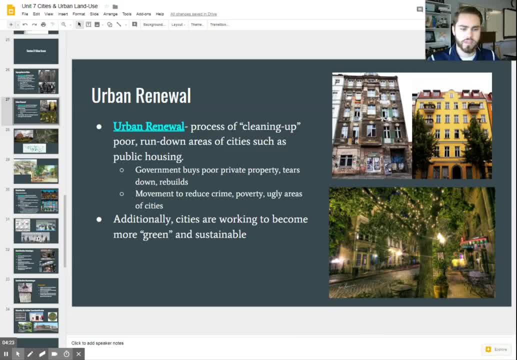 to a different area of town. so basically they tear down the old public housing in the inner part of the city and they move it to a distant or further out location and rebuild it. hopefully it's a lot nicer and it cleans up that area of town. businesses are gonna be more attracted now to that area if it's. 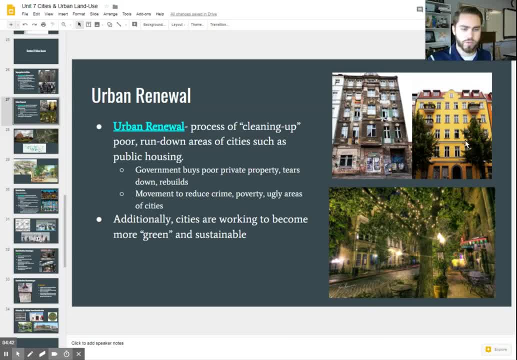 fixed up, it looks a lot better. you can see what it looked like before and after over here, and so businesses, you're gonna want to come back to that area, which previously was heavy crime and nobody wanted to be located there, and so we start seeing this, what we call urban. 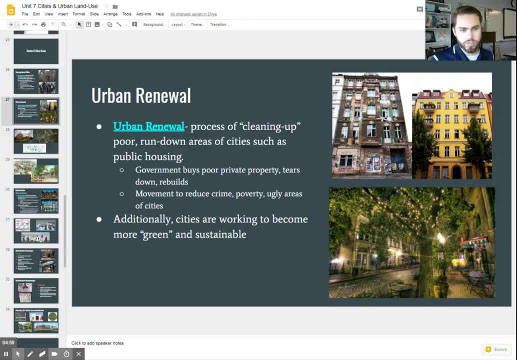 renewal and cleaning up the city's, the inner city, which had been long associated with. you know poverty and crime and you start seeing some improved. you know green space as well. cities are oftentimes seen as these hard concrete jungles. well, you know cities are working hard now to break that reputation and 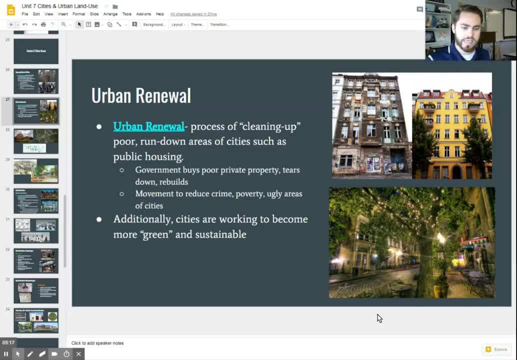 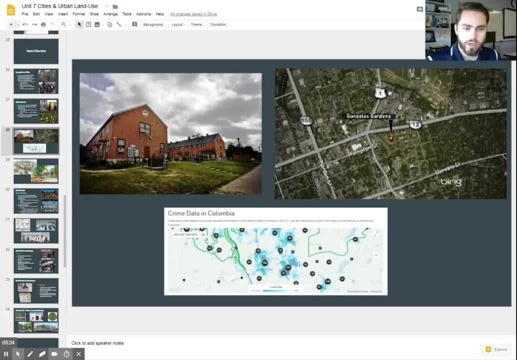 make it a more enjoyable, cleaner, greener place to live. you can see some of the images here of what cities are trying to do and what they're trying to do, and so here's a example in a local area here in Columbia that they are trying to renew. 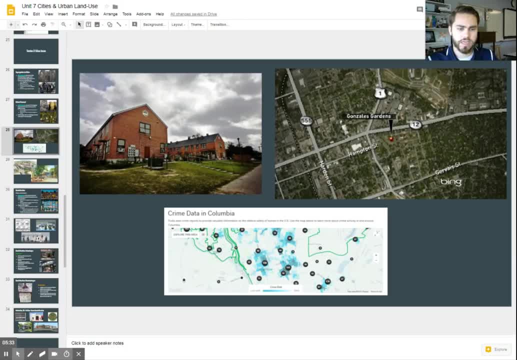 all right. so one of the housing projects downtown Columbia was called Gonzales Gardens and this area was known as a very crime-ridden area and your five points, you know. it ended up, because of that same type of problems with public housing that we talked about before, being the hotbed for drug dealing and 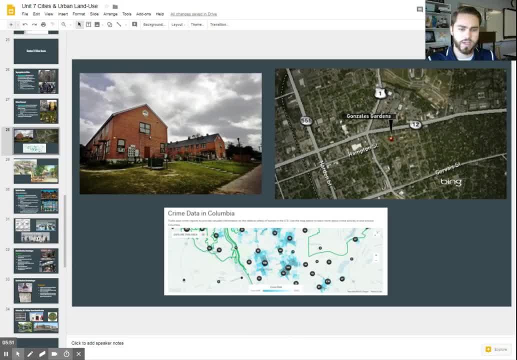 gang violence, and so we're going to talk a little bit more about that in just a minute. it's also in the outskirts of uptown Columbus. we see the residence process ready. it's about 22 states, and so we see a higher crime rate in that area. you know around that Gonzales garden public house, and so it's. 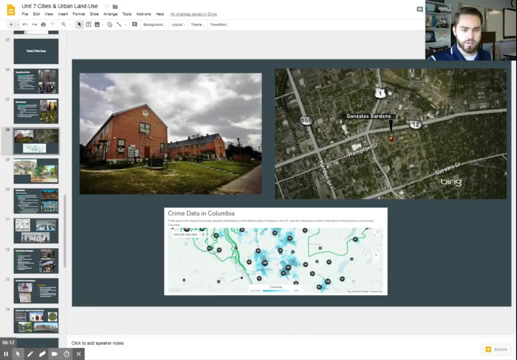 also very dilapidated. you can see what it looked like here. it wasn't very pretty. they ended up just they're in the process of doing this, currently tearing example here of, you know, an area that was previously very crime infested and and now making it a nicer place to be. so urban renewal- here's some other ways in. 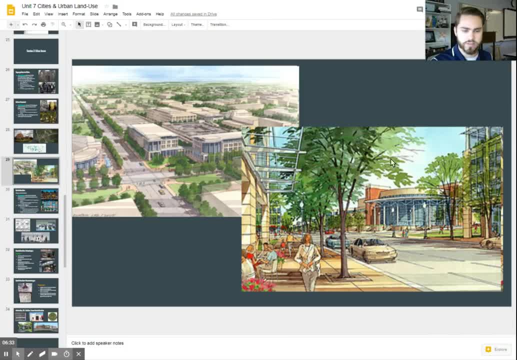 which Columbia is trying to improve its green space here you can see the Colonial Center or the basketball arena here and all the green spaces that they're trying to renovate in this industrial, former industrial area, and so this is something that many cities are trying to replicate around the world. 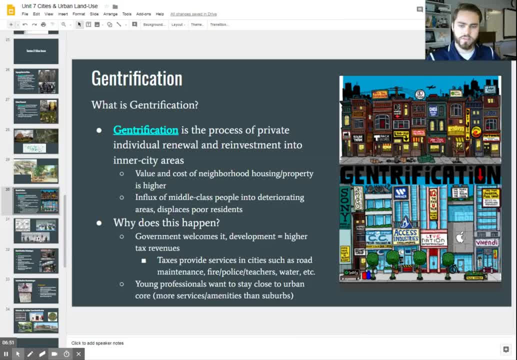 all right. another big issue focused in cities today is what we call gentrification. all right, so this is similar to urban renewal, the difference being that governments are usually ones cleaning out the cities, and urban renewal gentrification is when private individuals go into a bad neighborhood. 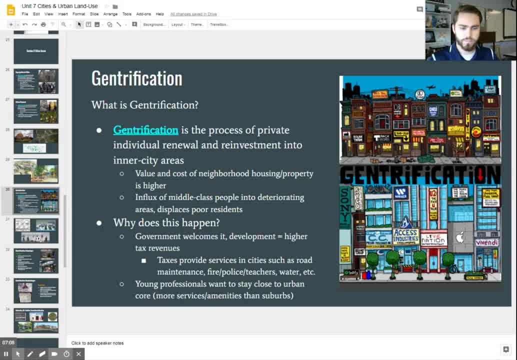 buy up the property, fix it up and make it a nice neighborhood. you can kind of see, based on this illustration here, an example of that. you know, when you have, you know, not as great housing, so so bad housing, and it's run down, you're not going to get the best. you know businesses to come in, there's not your. 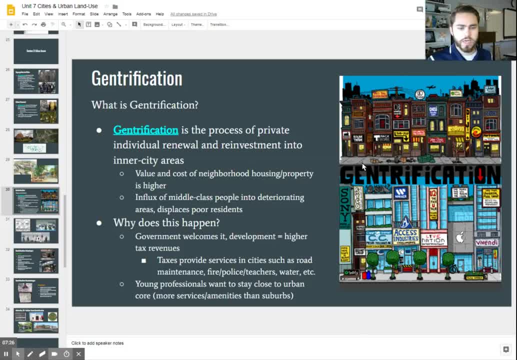 high-end businesses. when people come in there and buy up the property, fix it up, you're going to get better businesses, people you know that are. you know businesses that are going to cater to the middle class and and people that have more money than the people that used to live there, which were generally. 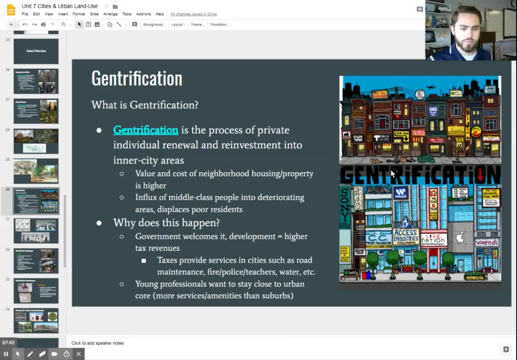 you know, poor and could not afford the spend money at some of these other businesses. so a lot of ways gentrification is a good thing. you know you buy up a piece of property, you make it better, you reinvest, it's a nicer piece of property. afterwards the value: 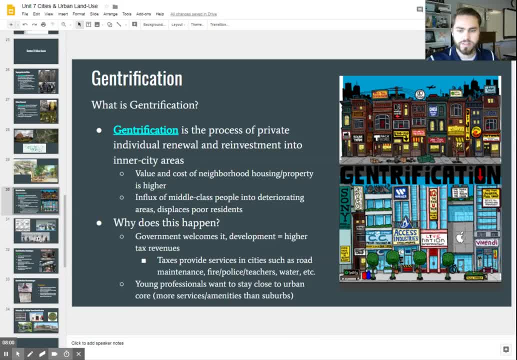 of your property goes up, the neighborhood becomes nicer, businesses come in, more middle-class people moving into the city. that's, it seems like a very good thing. this means higher tax revenues for the government. the city can fix its roads and, and you know, taxes are a big part of what. 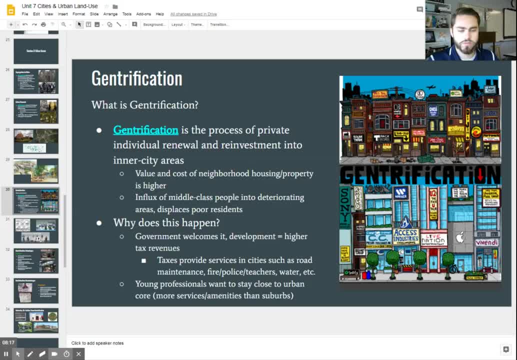 happens to paying for roads, for teachers, for firefighters, police, you know you have better quality of water and other things of that nature. so gentrification seems like a very good thing and we're going to talk about, though it's seen by many people as a very bad thing, so let's take a look at. 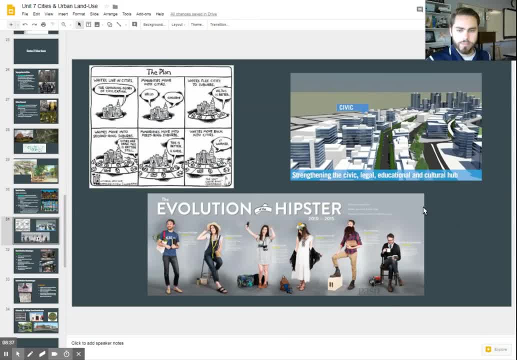 what this problem is. all right, here's a good example of the type of people that are moving into it. you hear the term hipster. all right, this isn't a big part of who's coming in, that these young professionals, these middle-class groups of people that are, you know, usually first fresh out of college, or you're. 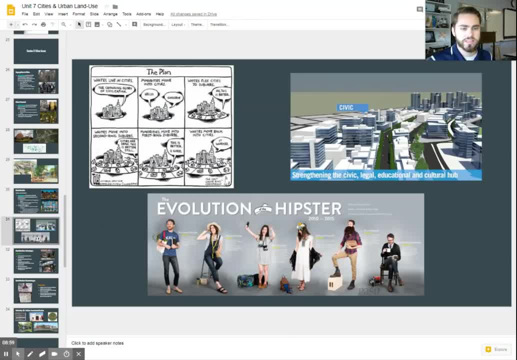 fairly young moving into the cities. you know they can't afford the nicest places downtown. so they take these you know used to be dilapidated poor areas and fix them up and then makes the rent go up, the price of the neighborhood go up there. all right, so some advantages obviously. 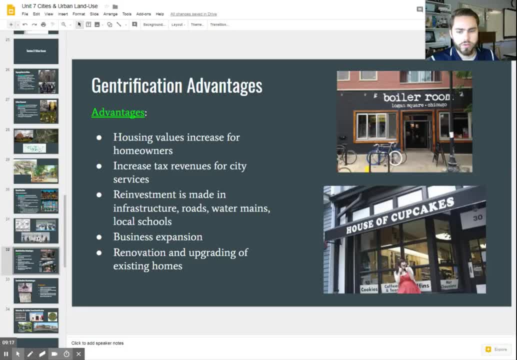 housing values are going to increase. you know your homeowner Association is gonna go up. you're gonna have nicer buildings than were there before. more tax revenue for the cities. they can use that money to reinvest into better roads and better infrastructure. you know, pay more for better police departments and 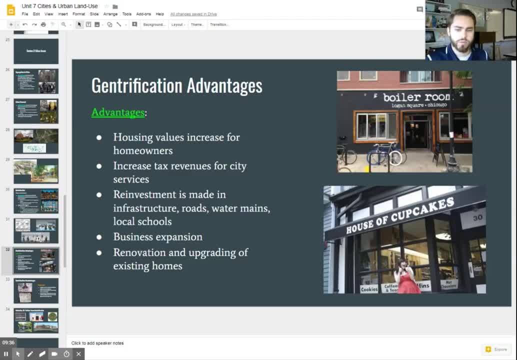 fire departments and teachers and things of that nature that taxes pay for, so they can reinvest a lot of that new tax money into the city. you have more business in there to, you know, cater to the, the people that are moving in there with more money than were there before, and they're renovating a lot of these areas. 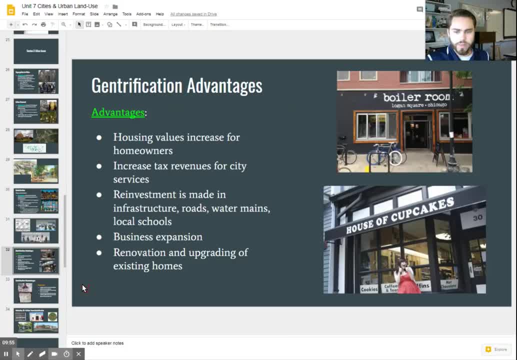 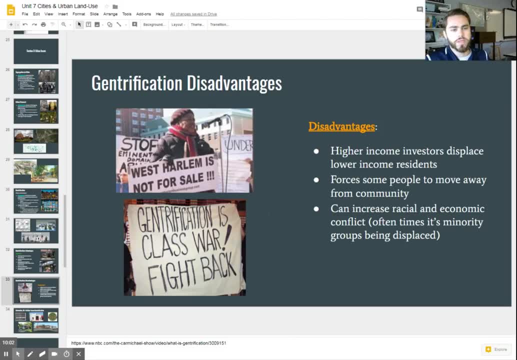 so it seemed as a very good thing by many people. however, there are some disadvantages. some disadvantages would include that the people that were living there before- so people were still living there before the gentrifiers came in- and what this does is to it displaces the people that live there afterwards, for 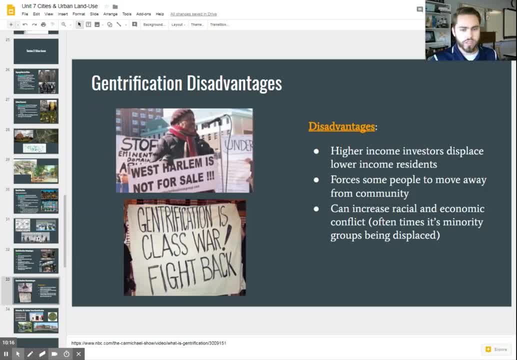 you know what you may say. why are they displaced? well, a lot of the people were living there, you know, in a very low rent area because that's what they could afford. when people come in there and fix up the neighborhood, these landlords are going to jack up the rent prices because people now want to pay more to live in. 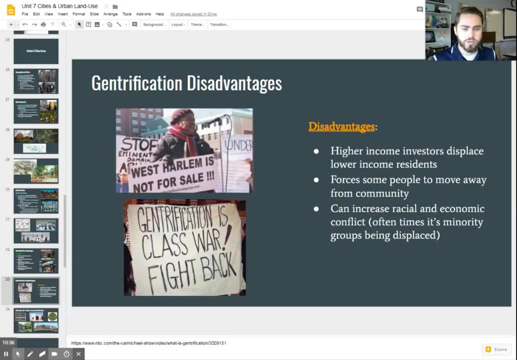 these areas. now that's getting fixed up and that's, you know, making to where the people that were renting the lower rent areas, when the rent becomes higher, they can no longer afford to live there and they're forced to move away from their- you know, their home, which you know. 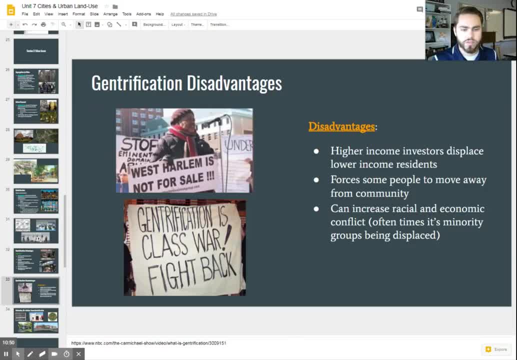 some people have lived there their entire lives and this, you know, really changes the community and it it seems like, in a lot of ways, class warfare, all right, where the middle class is taking over from the, the lower class, the people that can't afford as much, and oftentimes it's seen as a racial conflict as well. 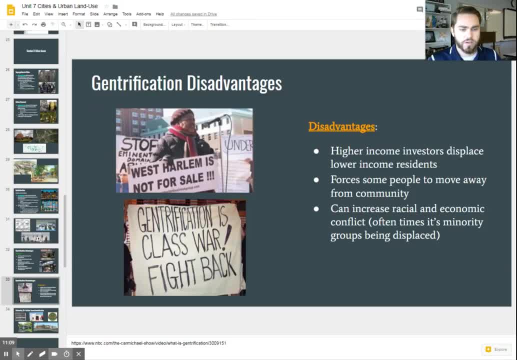 because many of the the residents are minorities that they're displacing, and most of the gentrifiers are of the white or white color. so they're they're- they're not majority in these cities, and so oftentimes it's seen as not only class warfare but also 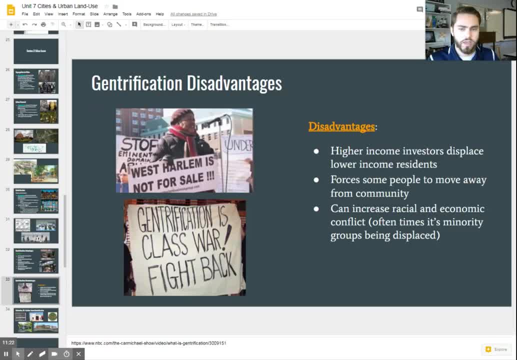 you know something, that's a racial divide and conflict as well. so gentrification. again, there are good things and bad things and there's different opinions on whether or not it should be allowed or not, but it is something important to understand. you'll see this a lot, you know in. 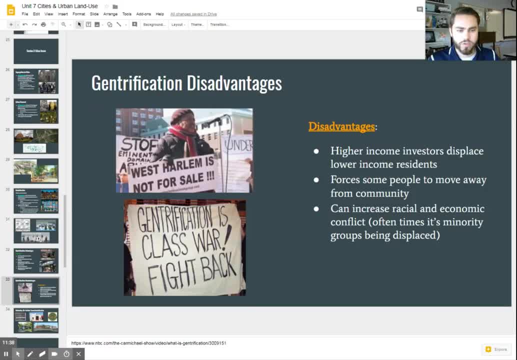 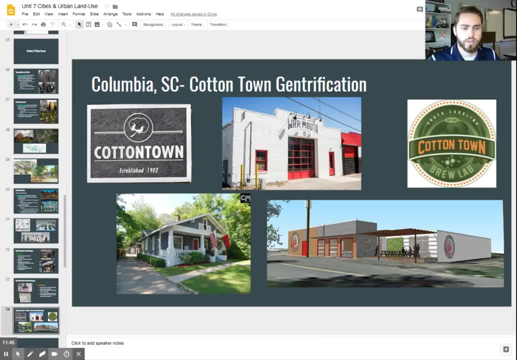 the news and in cities. if you go there, you can see areas where it used to be very bad if you go in, and now they're trying to fix it up. so you'd look no further than again in our you know city close by here in columbia, south carolina, cottontown is an area of downtown columbia where they are. 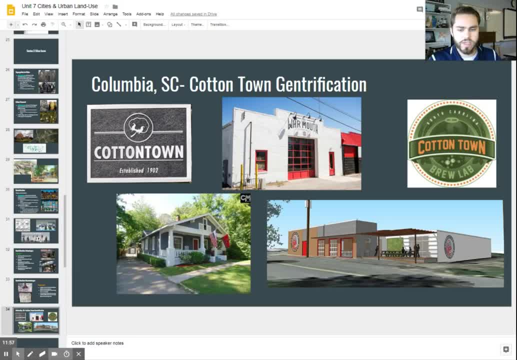 you know, focused on renewing that area through private investment. so people are buying homes that were run down and, you know, not so great, and fixing them up, making it a nice neighborhood and how it's one of the areas that is growing very fast. people are trying to move into cottontown. 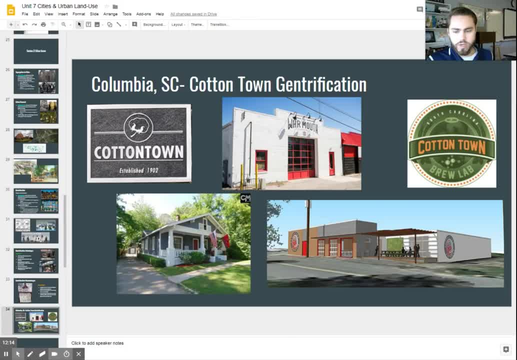 again where it used to be. you know an area that wasn't so great. you start seeing new businesses, such as this artisan restaurant. you know it's a little more expensive restaurant. you see a new brewery coming in there, something that you know is oftentimes following these gentrifiers to the 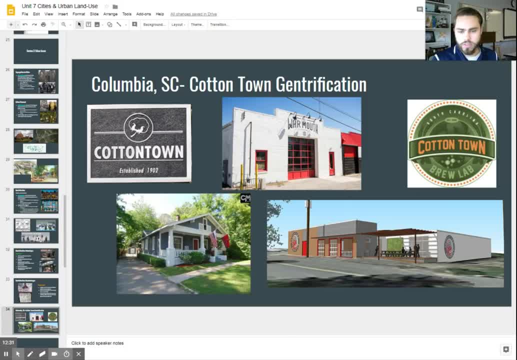 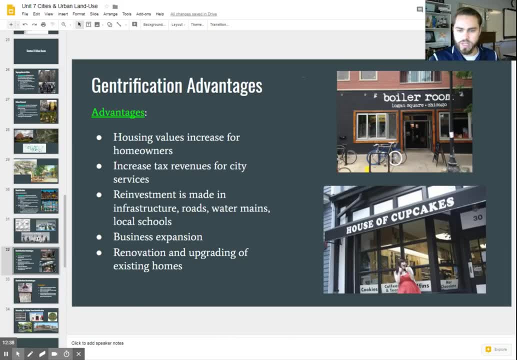 region, and so you can see that happening in our own backyard here in columbia as well. so gentrification: real quick review. it has its advantages increased. you have better taxes, you have better buildings. you can reinvest that money into the city, making the city a nicer place, but it displaces a lot of people as a result- the people that can't afford. 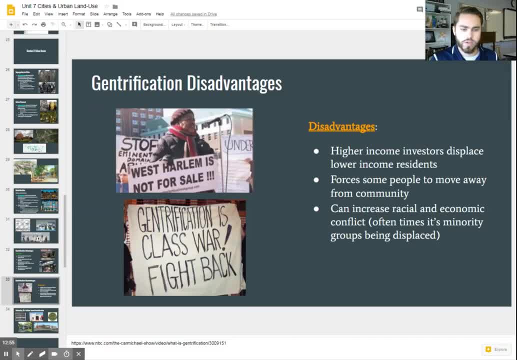 to live there anymore and it's causing many conflicts, not only of class warfare, but also conflict between racial groups. okay.